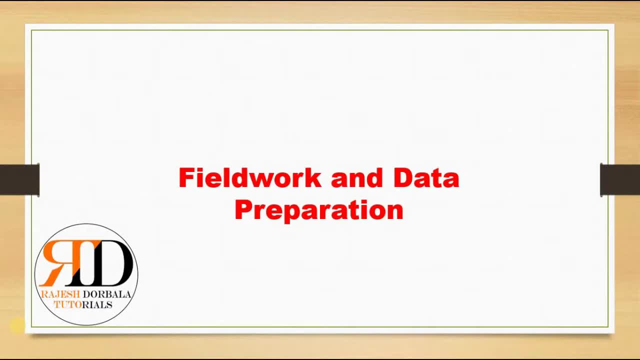 the evaluation of field workers And we are going to discuss the field work in context of international marketing research as well and identify the relevant ethical issues and explain the role of internet computers, the online research. So we are going to touch upon all the latest developments that are. 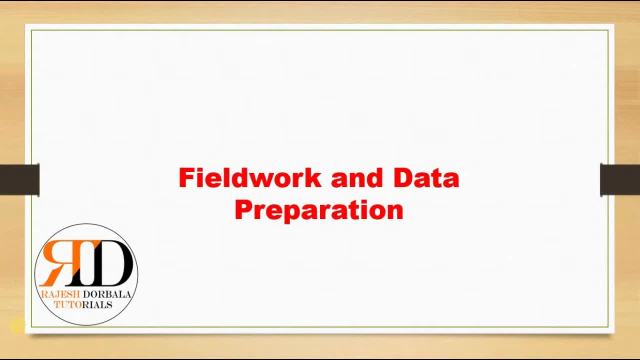 happening in this scenario. Before I go into the details of the chapter and what other important parameters that go into field work, own online survey on several platforms. obviously you must be using Google Forms, which can be used for surveys. there are other fields or other platforms where 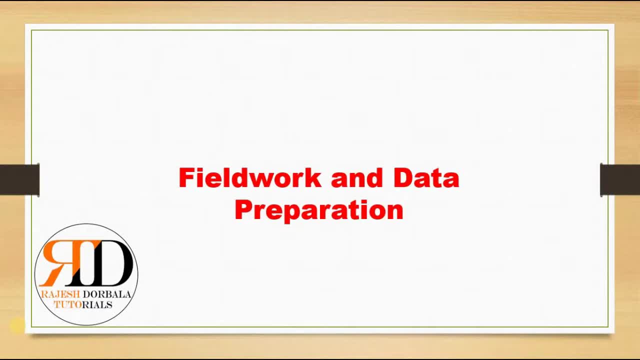 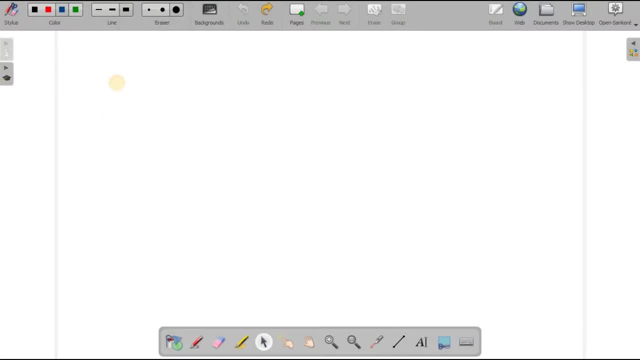 you can create, one of which is create surveycom. I will just write it over here so that you can use it. one is wwwcreatesurveycom. okay, so this makes it easy for you to understand. so here you can go and just create a survey for yourself that is on wwwcreatesurveycom. fine, there could be. 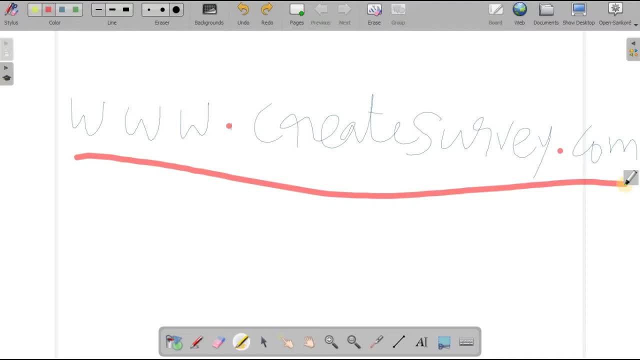 other platforms. for instance, let us say you can also use some platforms like zoomerangcom. okay, this is also a important tool. there is another, you know, market marketing tool, an internet-based company, technology enabled, full services marketing research company. that is markettoolscom. you can just. 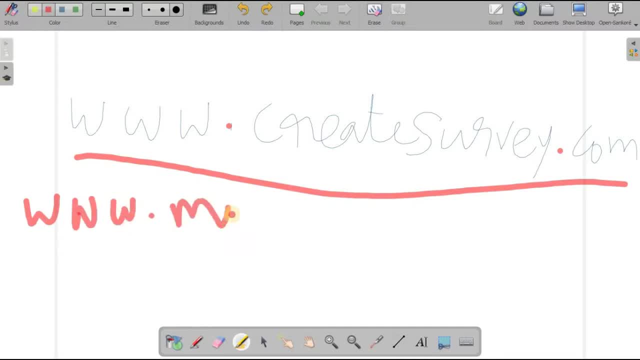 take it. wwwmarkettoolscom- fine, if you want, you can take this as well. zoomerangcom- okay. so these are some platforms where you can create, monitor, administer your own surveys. fine. so let's go back to our slides and we will study what the field work and data. 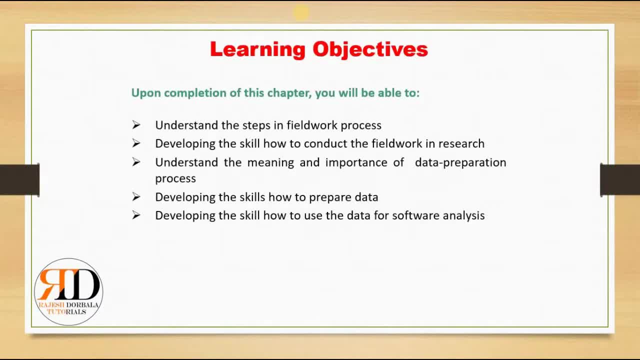 preparation process is. so, upon the completion of this chapter, or upon the completion of this lecture, you will be able to understand the steps in field work process, develop the skills how to conduct the field work in research. understand the meaning and importance of the field work process and how to conduct the field work in research. understand the meaning and importance of. 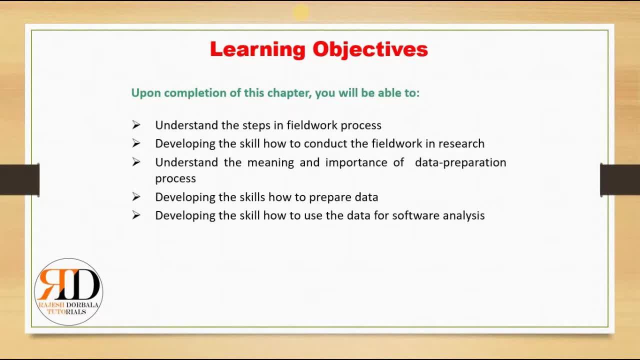 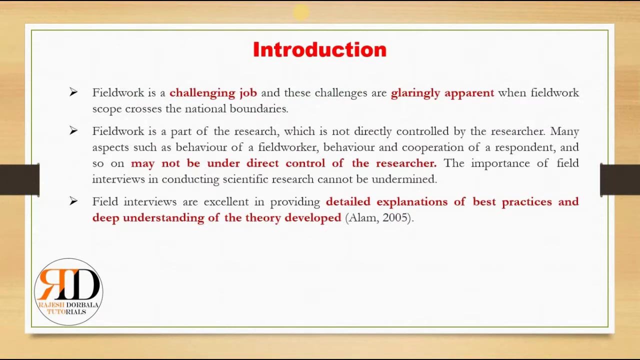 data preparation process, developing the skills on how to prepare data, developing the skills on how to use the data for software analysis. fine, so these are the various outcomes that I am expecting, so, by the end of this lecture, these are the five things that you can take away. so let's see, obviously, what we 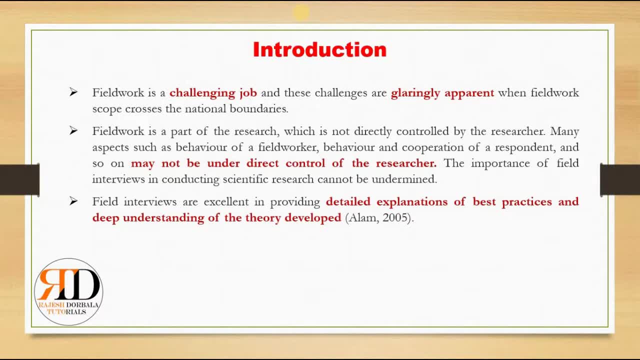 are talking about is a nature of field work. now the research is made a research. research is the nature of fieldwork. research is Within research, to use data as a tool. the Research data is rarely collected by persons who design the research. This is very, very important. 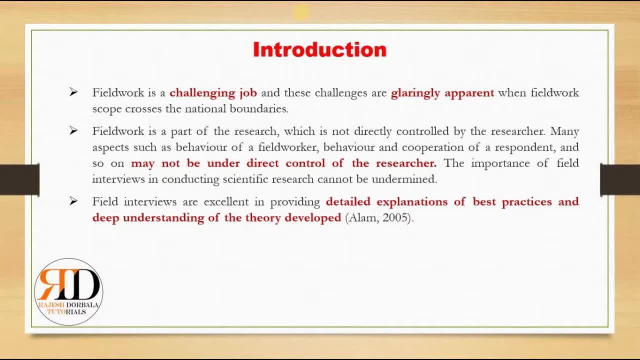 Those people who are conducting the research they rarely collect the data. Researchers have two major options for collecting their data. They can develop their own organizations or they can contract with a field work agency. In either case, data collection involves the use of some kind of field force. 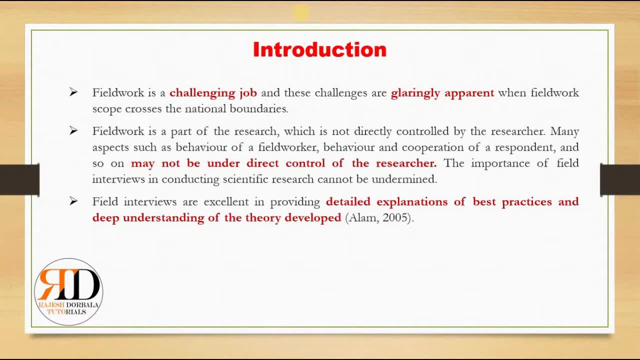 Now, the field force may operate either in field that is like personal, in-home or mall intercept, or computer email or internet survey. The field workers who collect the data, the field workers who are in fact collecting the data on behalf of the researcher, typically have little research background or training. 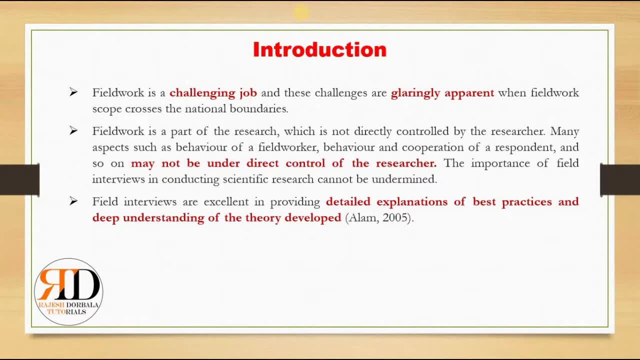 So whoever is collecting the data, we have to understand that they do not have much kind of an exposure to the training sorry research background. So the researcher have to be. the researchers have to be very careful in order to train them and give proper guidelines. 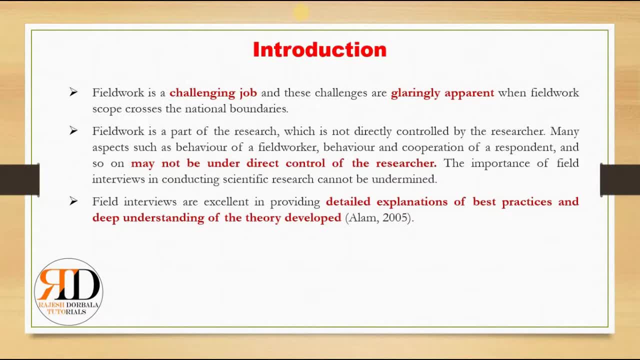 Now, more importantly, ethical concerns are also. you know they are also important. We have to take care of them. The researcher has to take care of the ethical concerns because the field workers are not aware of the research techniques and the background. They do not have relevant training in it, although there is ample opportunity for violation. 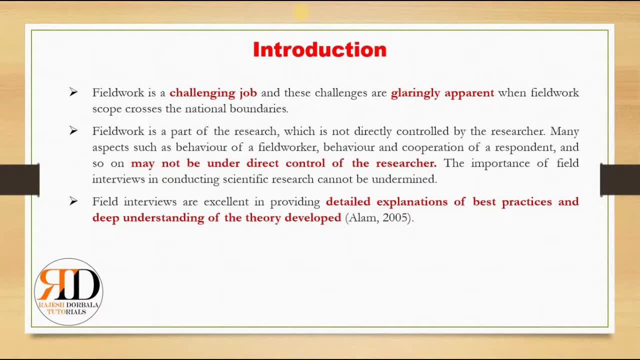 of ethical standards, clients need not be overly concerned with dealing with reputable field work agencies. Now you have to understand that here, as far as the field work is concerned, reputation again plays a very vital role. so if we are hiring some reputed agencies who do the market, 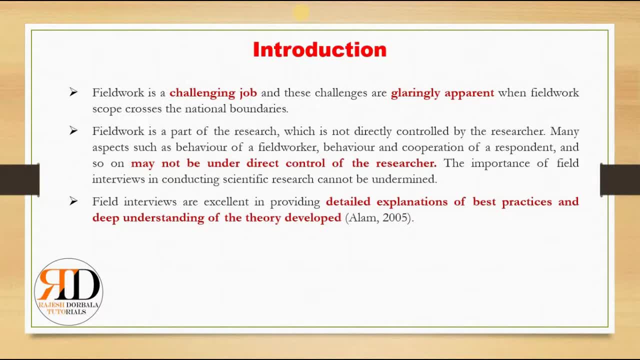 research for us, we don't need to worry about the ethical problems. Now, in words of Michael Reddington, who is a senior vice president for corporate development and marketing research counselors group, that is MARC group. you can visit their website also. that is marcgroupcom. 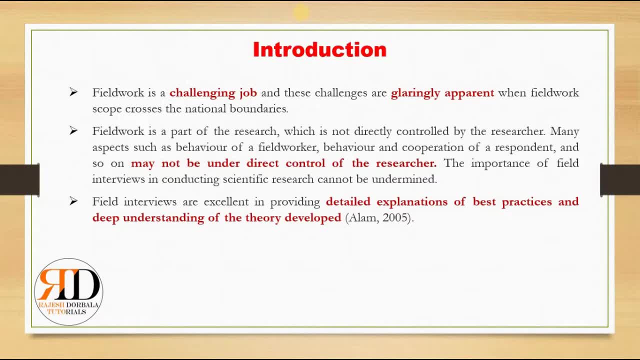 Now this guy, Michael Reddington, is an aggressive advocate of field quality. now his evaluation of the quality of field work in marketing research industry is, you know, to quote him. I would like to quote him as well. I was very pleased to help shoot down the myth that data collection is characterized. 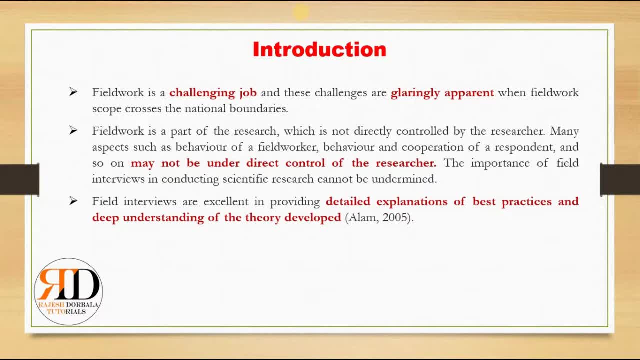 by a bunch of people out there attempting to bend the rules, to rip you off and to cheat on interviews. there are a lot of people on the client side who believe just that. quite frankly, we were out trying to find it but we didn't. that was a revelation to us. we 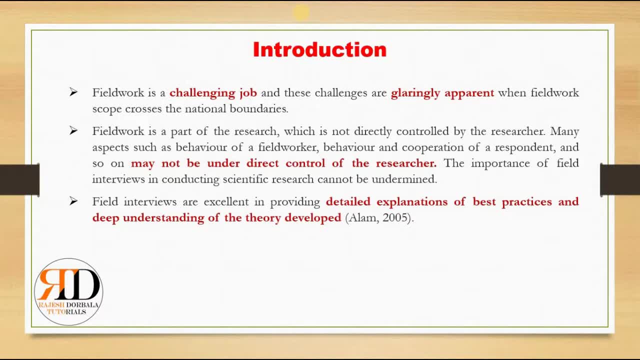 We were afraid that there were more unethical practices in the field than there really were. So the quality of field work is high because the field work, or data collection process, is streamlined and well controlled. So that is what the backdrop or the nature of field work is. 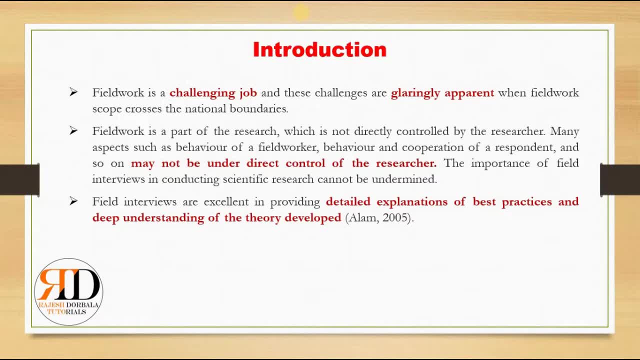 So we need to be very careful, because two things that come out for me, if you ask me two things, that is: one is the research. the person or the researcher is not the person who is collecting the data and the team or the field workers who are collecting the data. 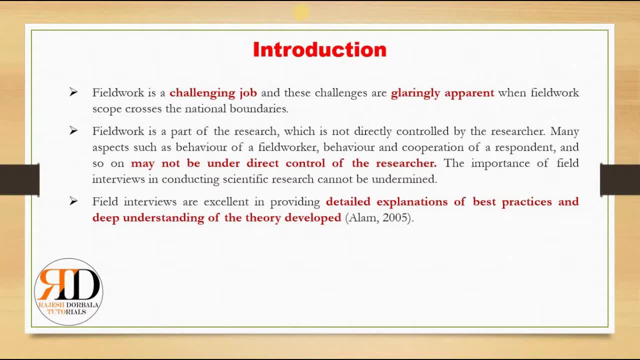 have little exposure to research knowledge. So the researcher has to take care of the training part and, moreover, the researcher has to take care of the ethical issues. So it is always advisable that a trusted, trusted agency should be entrusted upon with the task of collecting data in the field. 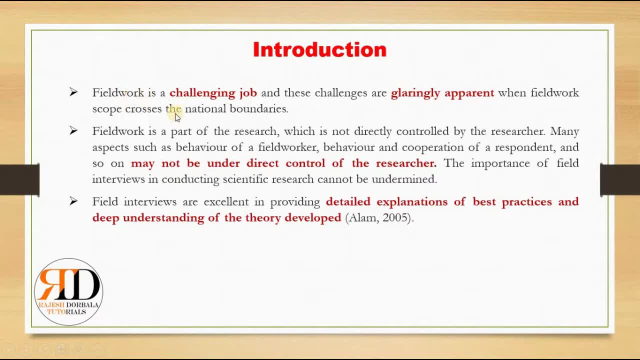 So that is the backdrop. Now let us see what I have written on the slides. that is, field work is a challenging job, and these challenges are glaringly apparent when field work scope crosses national boundaries. So it is challenging, that is fine, that is obvious, and field work is a part of research. 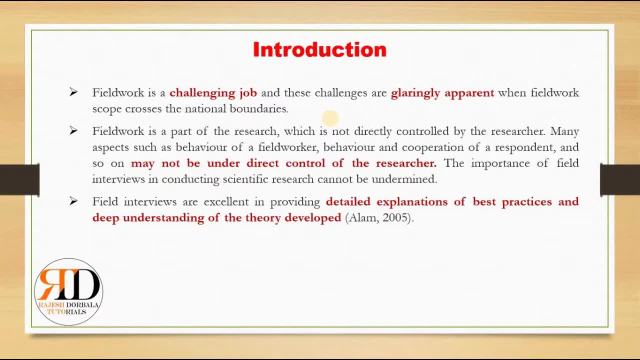 which is not directly controlled by the researcher. that is what I told you earlier. also, So many aspects of the behavior of field worker, behavior, cooperation of a respondent and so on may be, may not be under direct control of the researcher. fine, 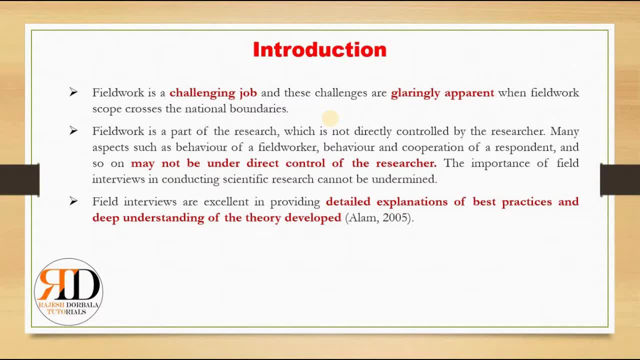 So the researcher has no control over the respondent. he cannot control the behavior of the respondent and he cannot even control whether the respondent would give responses or not. The importance of field interviews in conducting scientific research cannot be undermined again. So if I need to conduct a scientific research, the the you know conducting interviews. 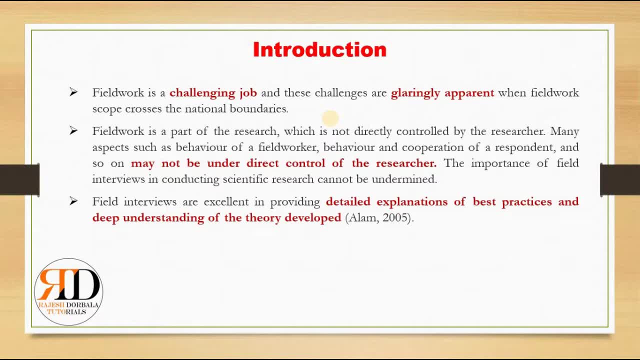 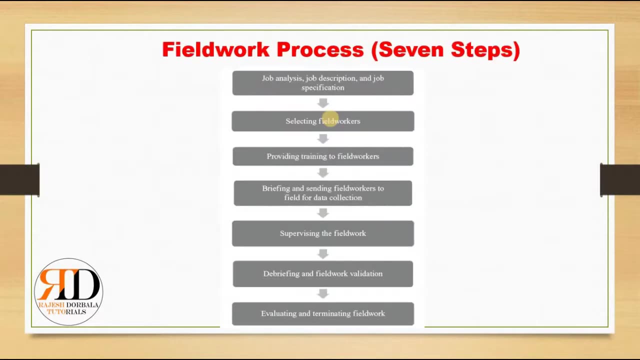 is of paramount importance Now. field interviews are excellent in providing detailed explanations of best practices and deep understanding of theory developed. This is what Alam in his renowned 2000 work quotes. Now the steps in research or the field work: One is job analysis. 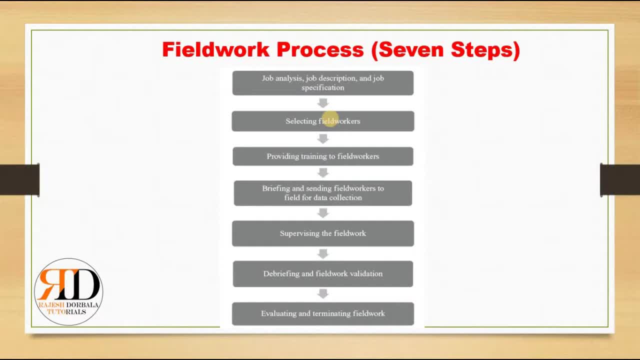 Job description and job specification. Okay, we will discuss all the steps in detail. You can pause the video and take down the steps. The first step is job analysis, job description and job specification. Number two is selecting the field workers. Number three: providing training to the field workers. 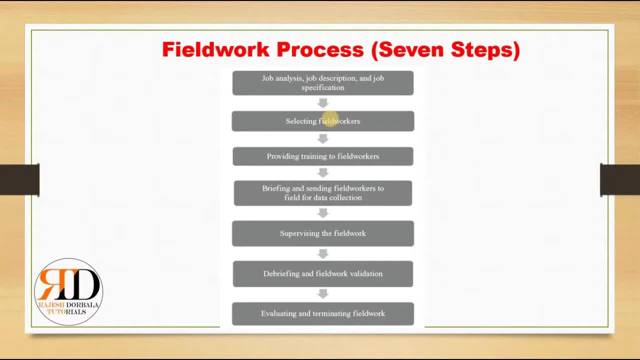 Number four, briefing and sending field workers to field for data collection. Number five: supervising the field work. Number six, debriefing the field work and validation. And number seven is evaluating and terminating the field work. Fine, So I am giving you seven steps, but if you see some popular research or popular literature, 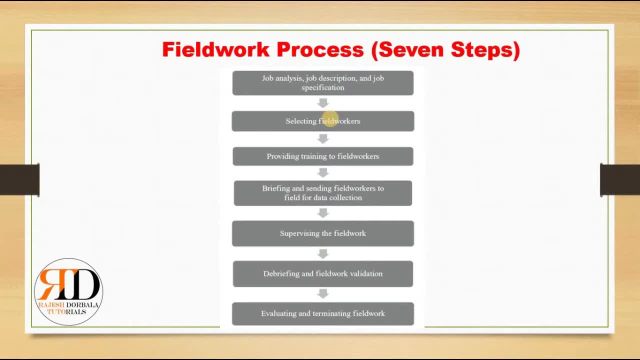 available in the market, some books. they give only five steps. okay, So the steps could be: number one could be selection of field workers. Number two could be training of field workers. Number three, supervision of field workers. Number four: validation of field work. 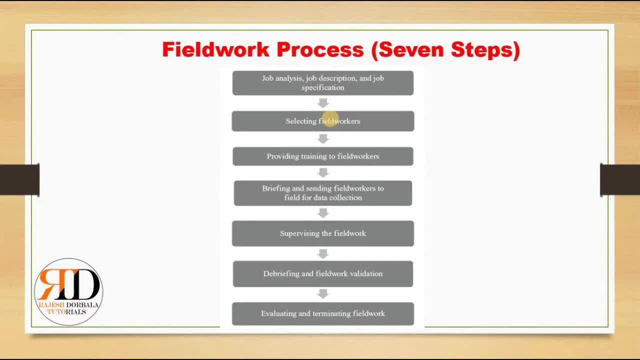 Okay, And number six is evaluation. sorry, number five is evaluation of field work. So usually in books they give only five steps. I have added a step before. that is job analysis, job description and job specification. okay, And then the other thing that I have added is briefing and sending field workers to the 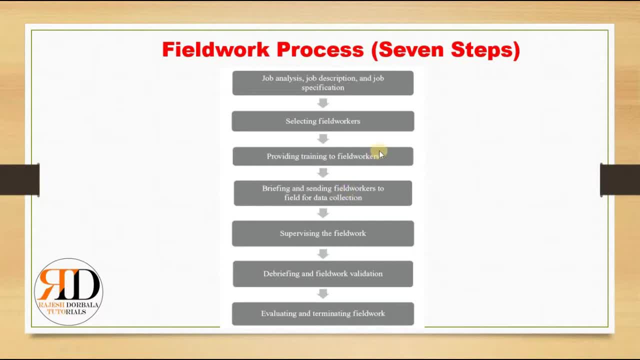 field for data collection. So, if you want, you can remove these steps, Step number one and step number four, from the seven step process and just you can have these five steps for your answer or for your knowledge. Fine, So let's move and let's see. 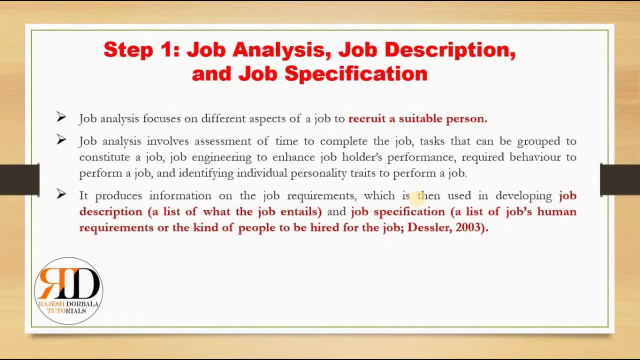 First one is job analysis, job description and job specification. That is, once I analyze the job and I get to know what the job consists of, it helps me hire the appropriate people. Okay, So I can look for the agency or the field workers who can collect data for me. 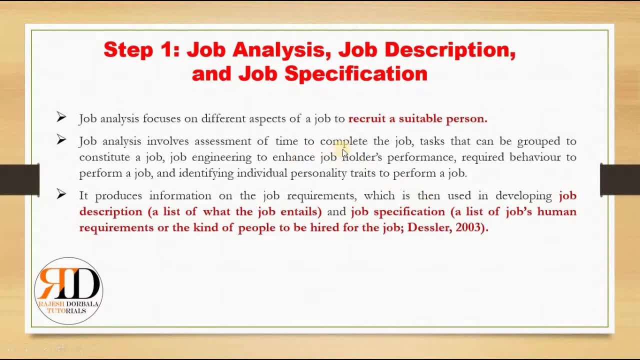 Now, job analysis involves assessment of time to complete the job, task that can be grouped to constitute a job. job engineering to enhance job holder's performance, required behavior to perform a job and identifying individual personality traits to perform the job. To put it simply, I need to do a detailed analysis of job. 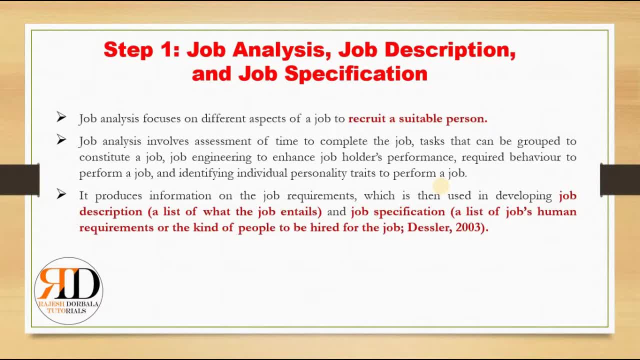 What goes into a job, that is to say, I need to create the minute milestones which could be achieved within that job. number one. Number two: I need to you know, analyze and come to a conclusion. when can this job be? 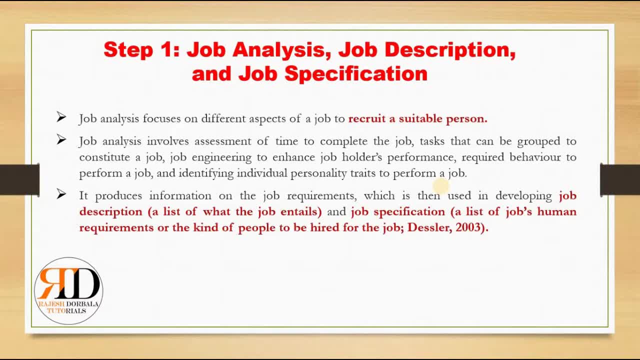 done or what are the timelines of this job? Number three could be: what are the performance parameters that are? you know that helped me analyze and evaluate the performance And could be like I need to know what kind of a behavior is required for this job. 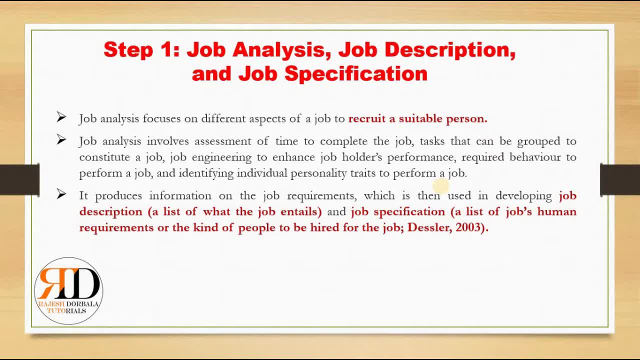 So I need to go deep into this job and make detailed notes or detailed guidelines so that it becomes easy to train the field workers and, at the same time, it also becomes like I can give them a standing operating procedures- SOPs- to my field workers. 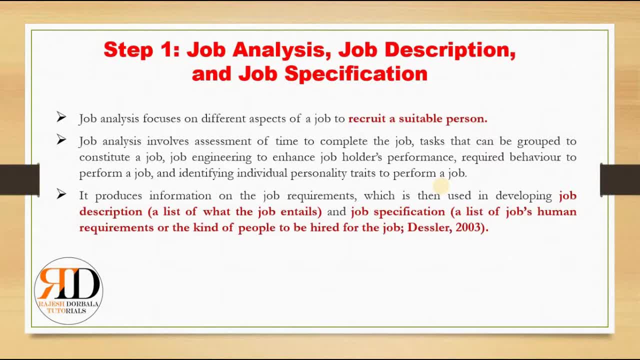 Okay. So for that reason, analyzing the job, Describing the job and giving job specifications is of paramount importance, because this renders objectivity to the field workers. And the last point: it produces information on the job requirements which is then used in developing job description. 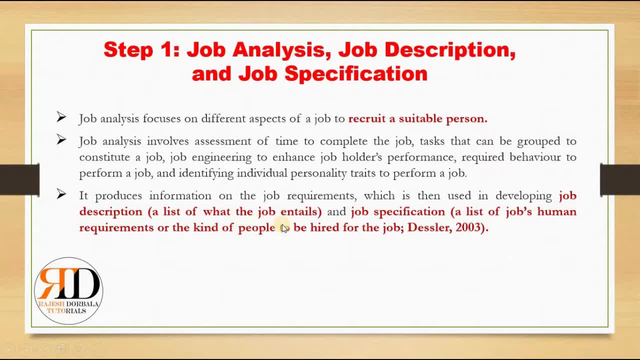 That is a list of what the job entails. That is what does the job ask you to do. And job specifications: That is a list of jobs, human requirement or the kind of people to be hired. That is what Desler said in his renowned 2003 work. 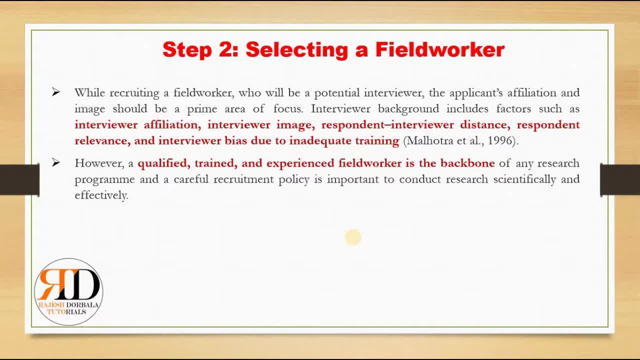 Now, second step, that is, selecting the field workers. So when you are selecting the field workers, the researcher should develop the job specifications for the project, taking into account the mode of job or mode of data collection. Okay, Very, very important that the researcher is clear about the job specifications so that 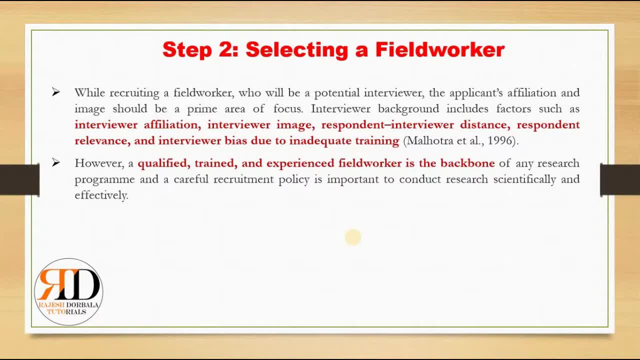 it becomes easy for him or her to understand how the data would be collected and then describe what characteristics the field workers should have. Okay, So based on this, he should make a note that these are the characteristics that a researcher or the field worker should have, and then recruit appropriate individuals. 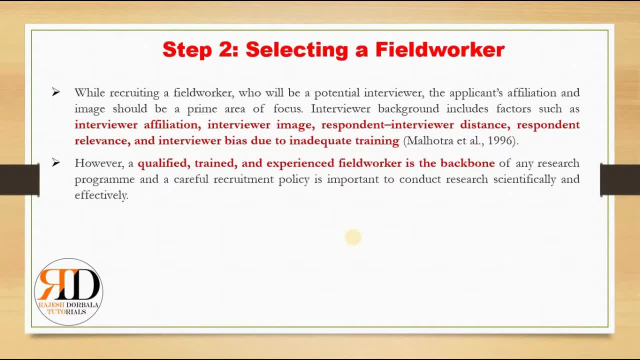 Okay, So interviewer's background characteristics, opinions, perceptions, expectations and attitudes can affect the respondents of the affect the responses they elicit. Okay, So it is very important to know that the kind of people I hire, their opinions, their behavior. 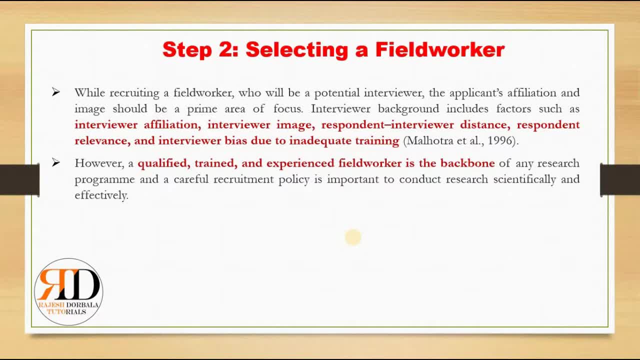 their perception, their views, their body language, everything can affect the responses of the respondent. So, while we are selecting the field workers, these things need to be of need to be taken care of And, for example, let us say, the social acceptability of a field worker to the respondent may affect. 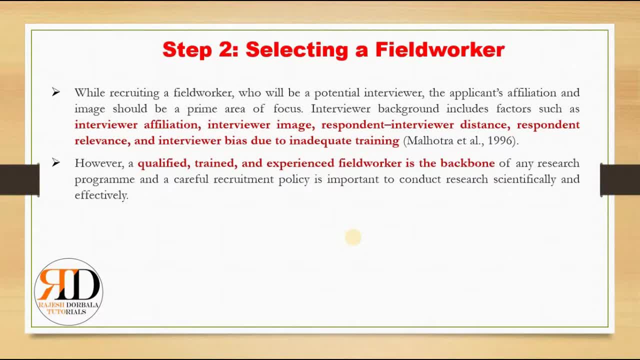 the quality of data obtained, especially in personal interviewing. Now, researchers generally agree that the more characteristics the interviewer and the respondents have in common, the greater the probability of successful interview. Okay, Okay, Okay. So if I hire the field workers who are not sophisticated or they are not suave, they 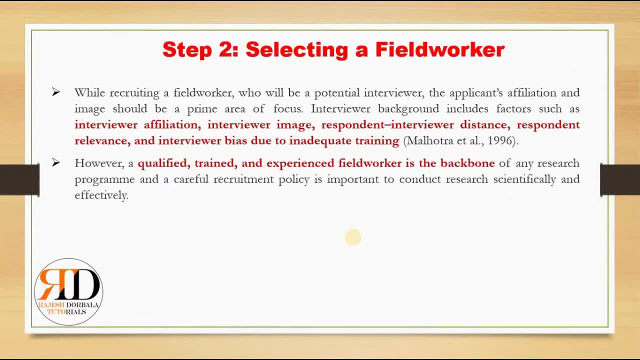 are not clean, they are not sophisticated, or maybe I could say they are not presentable. and if I send these kind of researchers to HNIs, okay, like high net worth individuals, So what happens? Okay. So the problem is, if these people meet the HNIs, there is very less thing in common. 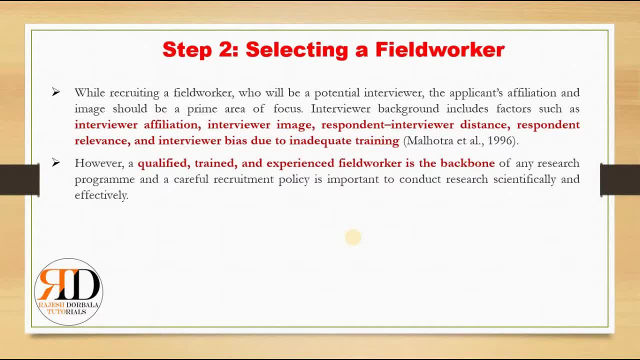 So the probability of the interview going successfully is very less. The respondent may not like to answer to such people and at the same time these field workers may not even get appointment from such HNIs to conduct an interview. So one thing is of very important: 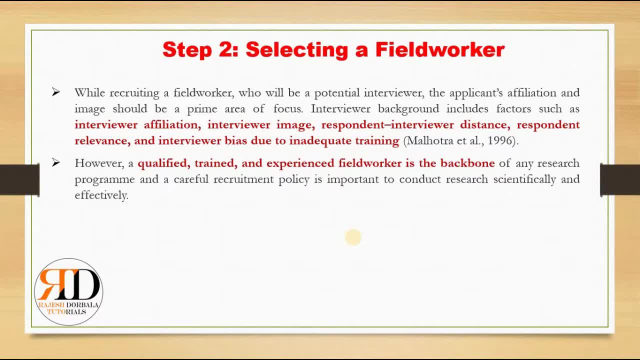 One thing is very important: that while I am hiring the field workers, I need to understand, or I need to see that the kind of people or the segment of my respondents. I should know what their profile is and then I should hire field workers who share similar attributes. 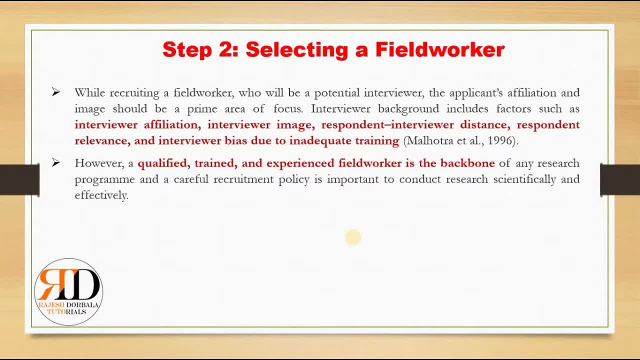 to those people in my segment. Okay, So there would be. When I do this, Okay, The chances of the interview going successfully is very high, Okay. So while recruiting a field worker who will be a potential interviewer, the applicant's affiliation and image should be a prime area of focus. 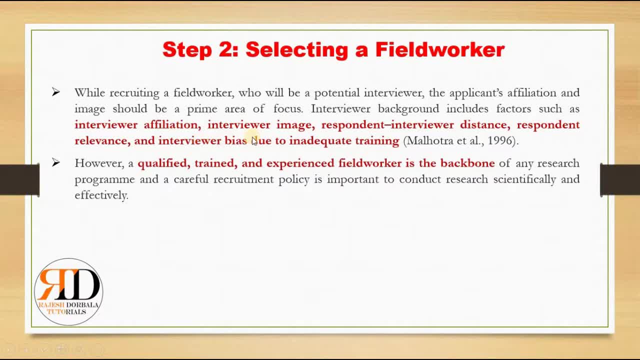 Interviewer background includes factors such as interviewer's affiliation, interviewer's image, the respondent interviewer distance, respondent relevance, the interviewer bias due to inadequate training, all these Okay. So this is what Professor Naresh Malhotra said in his work in 1996.. 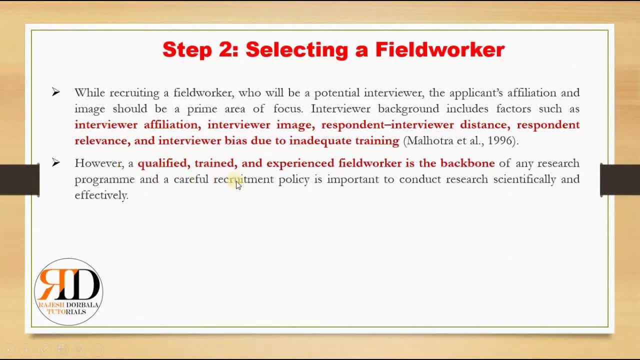 Now, moreover, however, a qualified, trained and experienced field worker is the backbone of any research program, and a careful recruitment policy is important to conduct research scientifically and effectively. Fine, So, overall, we need to hire people who do not have bias, who do not have, who are neutral. 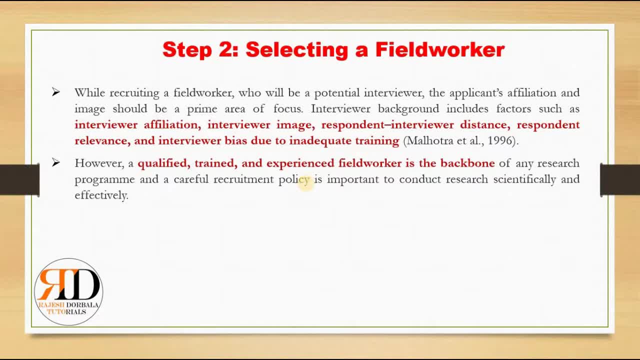 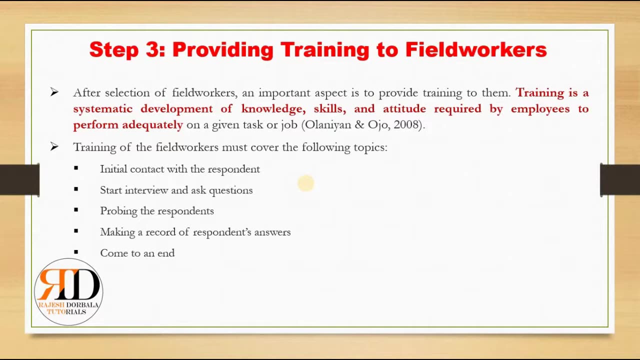 and share a lot. Okay, Share a lot of attributes which are similar to the respondents. Fine, That may help you in getting your interview successfully. Then, providing training to the field workers. Now, how do I provide training to my field workers? 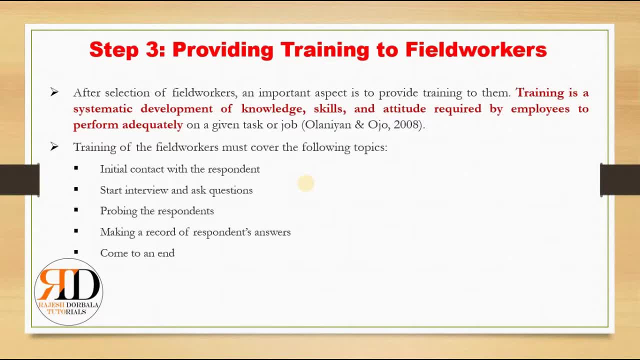 That is, once I have selected the required field. workers training again is a very, very important thing. Okay, I have to develop a systematic program through which I could impart knowledge, skills and attitudes required by employees to perform adequately on a given job or task. 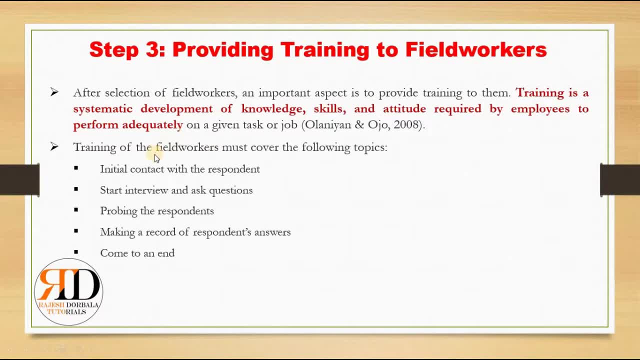 Fine. So likewise, training of field workers must cover the following topics, that is, initial contact with the respondent, start interview and ask questions, probing the respondent, making a record of respondent's answers And come to an end. So the researcher has to train the field worker on all the aspects and take them through. 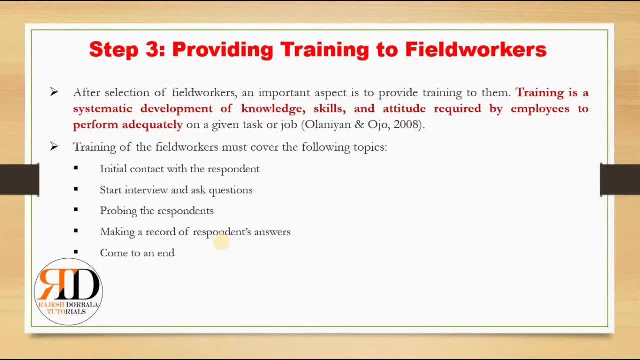 each and every step, meticulously handhold him, so that they get the clarity on what is expected from them and what should be the ideal outcome of every interview they conduct. So you know, both the researcher and the field worker should be on the same page. 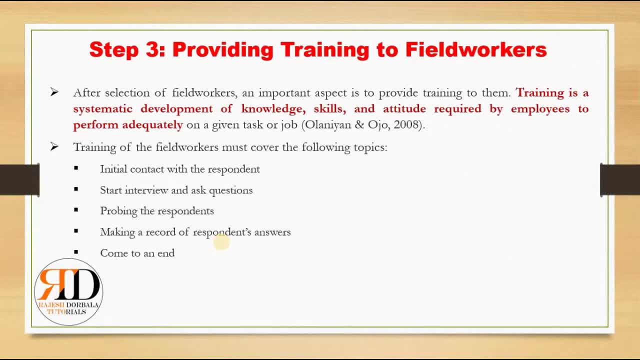 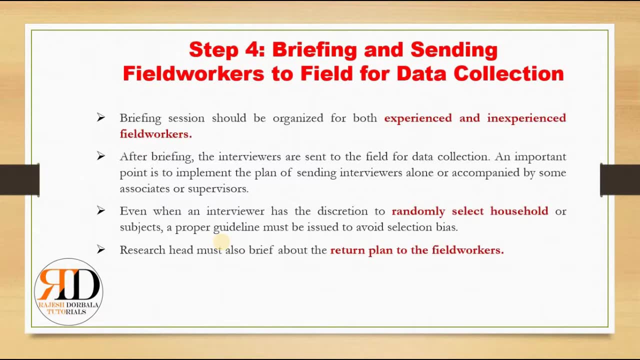 Okay, The field workers need to be clearly aware of what the researcher is expecting from them. Then step four, that is, briefing and sending field workers to field for data collection. Now, in this step, this I could say: this is just a. you know, you could avoid this. 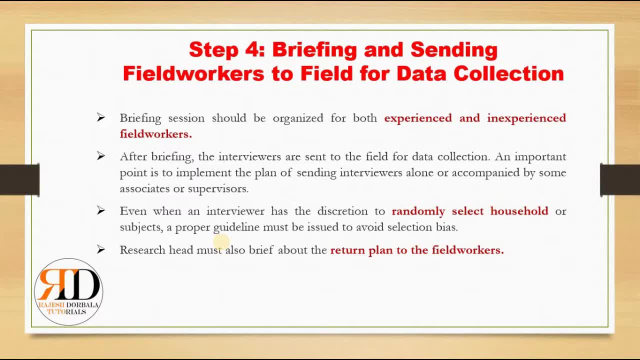 step as well, because most of the books or the literature available doesn't include this step. But just you know, there could be some loose ends which I would avoid. Okay, So there are some loose ends which I wanted to cover in this step. 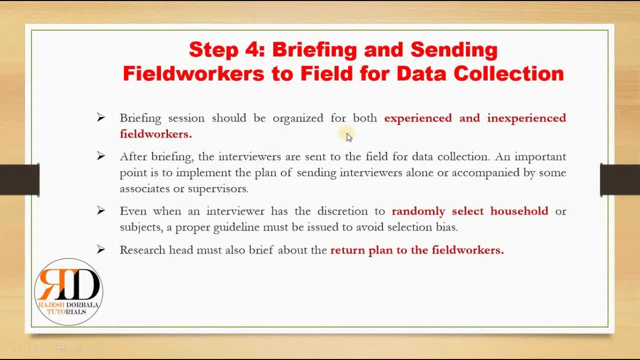 Now let's see. Briefing session should be organized for both experienced and inexperienced field workers. After briefing, the interviewers are sent to the field for data collection. An important point is to implement the plan of sending interviewers alone or accompanied by some associates or supervisors. 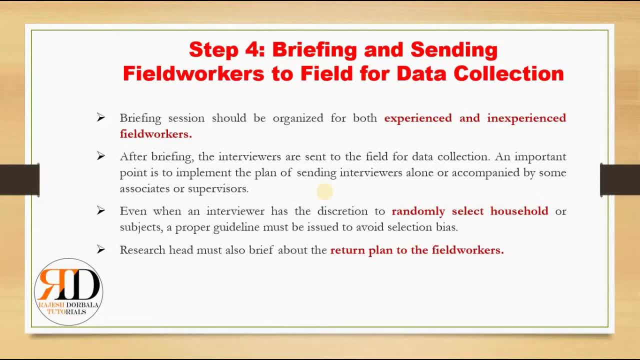 Now, even when an interviewer has discretion to randomly send interviewers to the field as discretion to randomly select households or subjects, a proper guideline must be issued to avoid selection bias. Fine, So though I can give, this is important. okay, because though I can give a lot of independence. 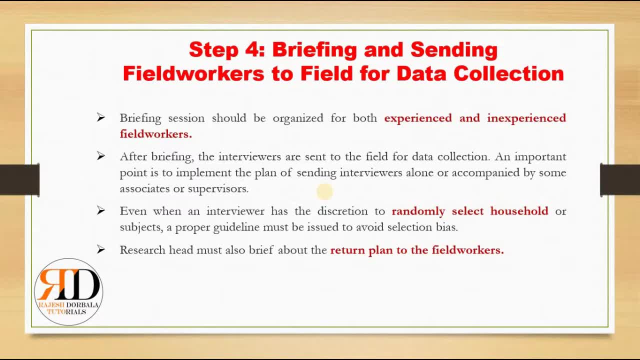 or autonomy to my field workers. but there is a possibility that the field worker, in order to reduce his workload, may you know, resort to selection bias. He may pick up respondents if let's say, for instance, this is a door-to-door interview. 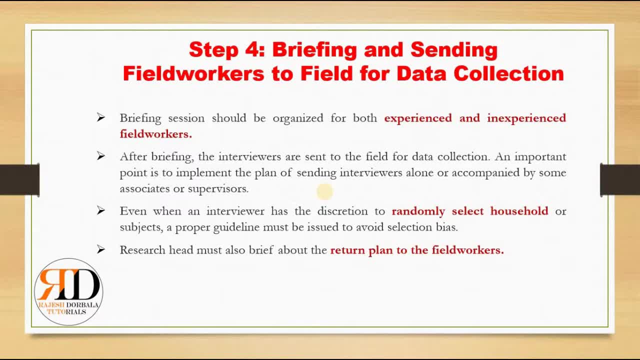 So in order to reduce his workload- or his, you know- to make his work convenient, the field worker could pick up respondents from any nearby locality and cover the number of respondents. So these kind of unethical practices can hamper the quality of the interview. 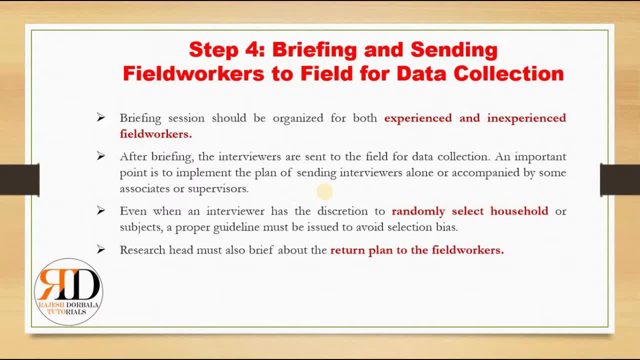 So this is the real spirit of research. So for this purpose proper guidelines must be issued. Then research head must also brief about the return plan to the field workers. So they need to be very clear how they are going to come back and what they are going. 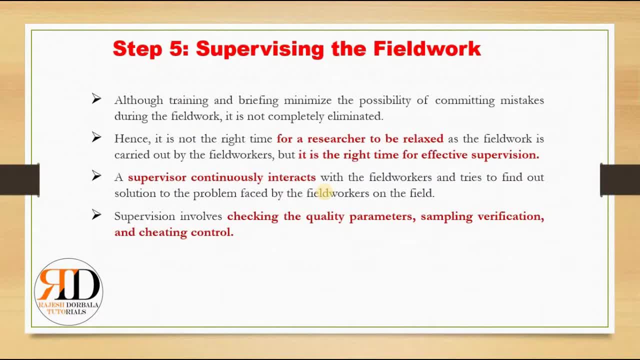 to bring back. And fifth step is supervising the field work, Although training and briefing minimizes the possibility of committing mistakes during the field work, but it's not completely eliminated. So I have trained my field workers, I have given all the necessary guidelines and I may be expecting that there wouldn't. 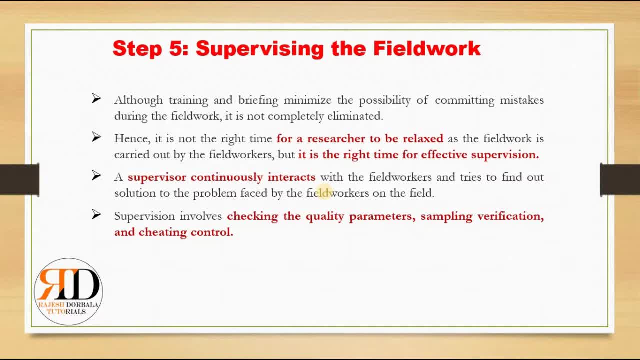 be any errors, but you cannot leave things to chances. You need to keep a tab on what's happening. That's what is step number five. Hence, it is not the right time for researcher to be relaxed, as the field work is carried out by the field workers. 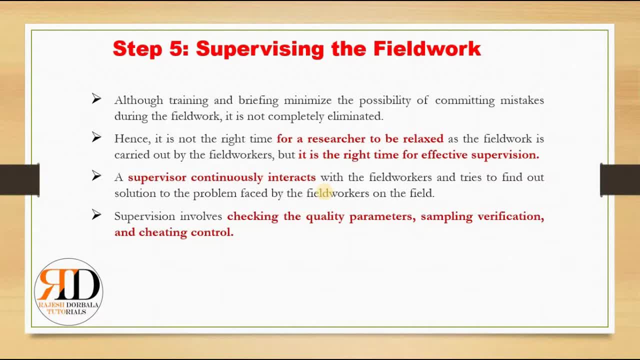 But it's the right time for effective supervision. A supervisor continuously interacts with the field workers and tries to find out solutions to the problems faced by the field workers on the field. Now it could be possible that our field workers- they are in the field, they are meeting the 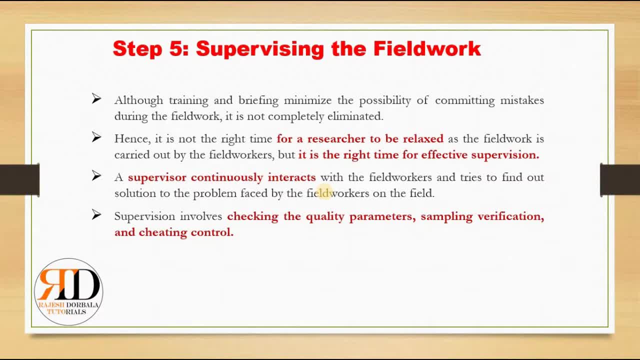 respondents and there could be some problem with the instrument, There could be some problem with the questionnaire, There could be some problem, Uh, But in selection of the respondents. So once the supervisor or the researcher is constantly monitoring what's happening in the field, it becomes easy, for it becomes easy for us to, you know, gauge the real responses. 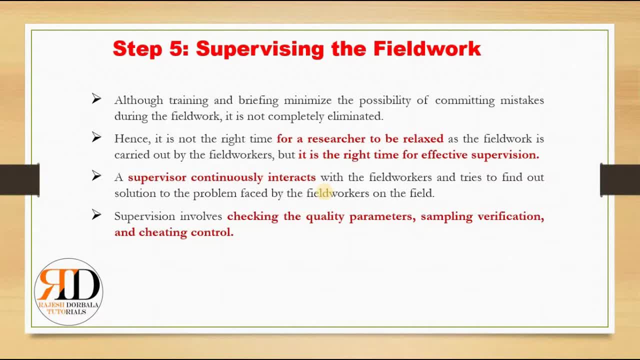 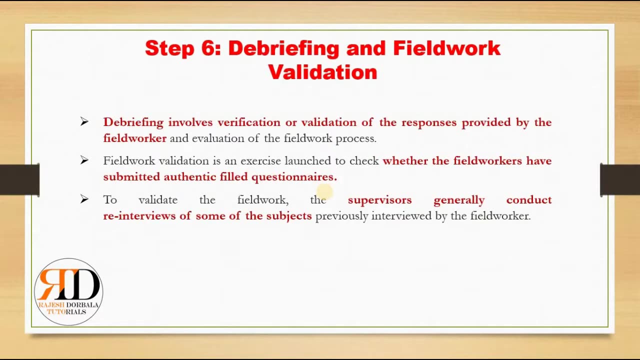 or the way the interviews are going on, and make any modifications or alterations before it's too late Now. supervisor, or supervision involves checking the quality parameters, Sampling verifications and cheating controls, Then debriefing the field work: validation. This is the sixth step. 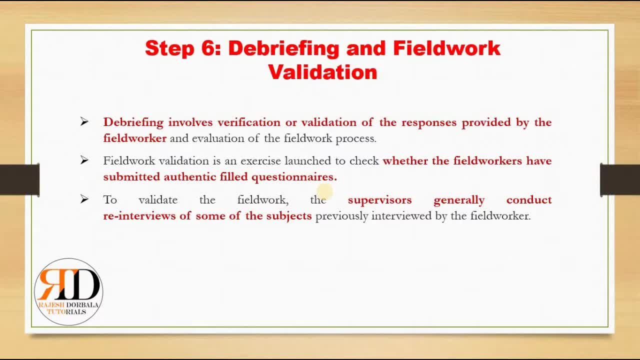 Now debriefing involves verification or validation of the responses provided by the field workers and evaluation of the field work process. This is quite obvious. Now, simply, you verify and validate whatever work they have done. You verify its authenticity, accuracy and all. 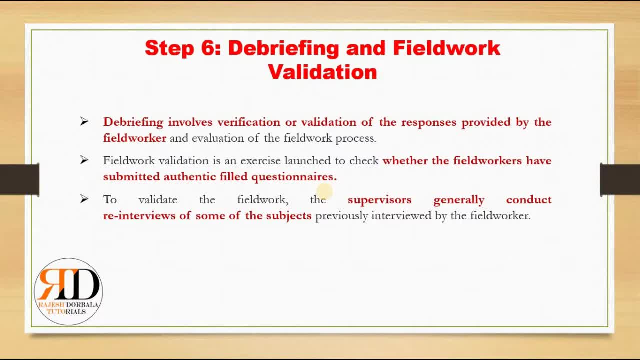 Field work. validation is an exercise. Validation is an exercise launched to check whether the field workers have submitted authentic field questionnaires. To validate the field work, the supervisors generally conduct re-interviews of some of the subjects previously interviewed by the field workers. 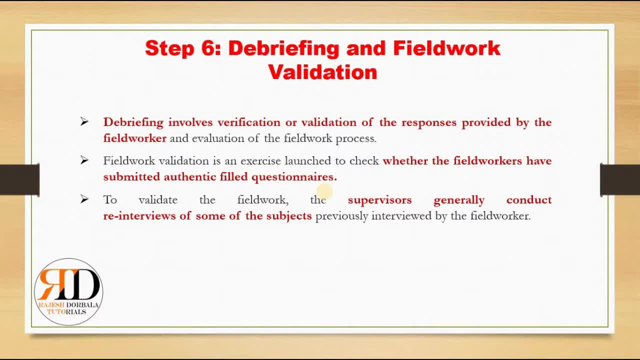 Fine, This is again quite self-explanatory. This is simply like cross-checking. My field workers have interviewed some, I randomly pick up some of the respondents and just cross-check. Fine, That's what is validation. And step seven: evaluating and terminating the field work. 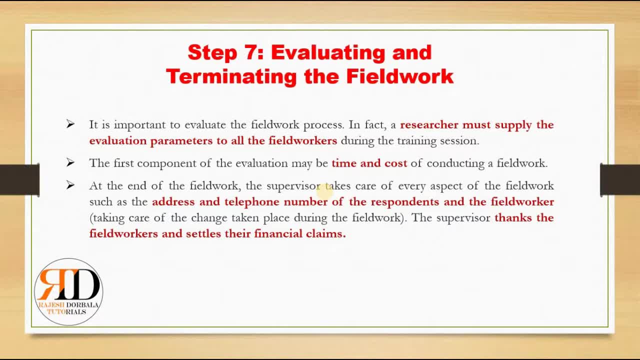 Now it's important to evaluate the field work process. In fact, the researcher must supply the evaluation parameters to all the field workers during the training session itself. They need to know on what parameters their work would be evaluated. Then the first component of the evaluation may be the time and cost of conducting the field work. 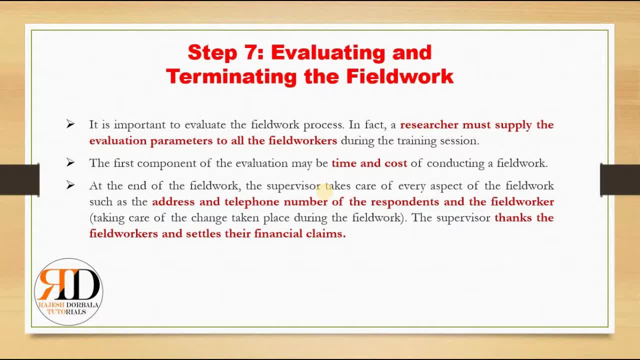 At the end of the field work. the supervisor takes care of every aspect of the field work, Such as the address and telephone numbers of the respondents and the field worker, taking care of the change taken place during the field work. Now the supervisor thanks the field workers and settles the financial claims. 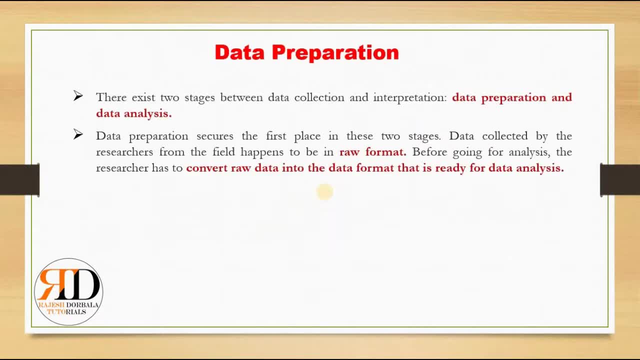 Fine, So end of the contract Now. once the field work is over, now comes the process of data preparation. Now my field workers have brought me the data. I have to work, clean and prepare the data for analysis. There are there exists two stages between data collection and interpretation. 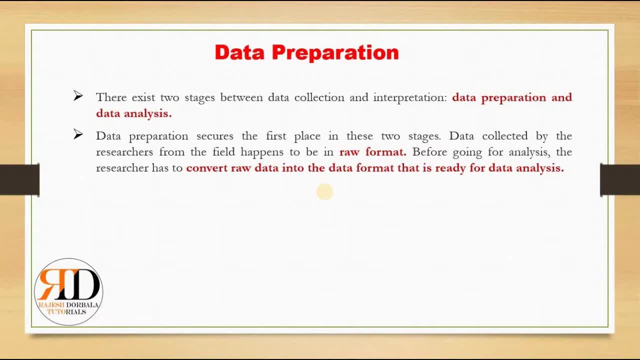 That is, data preparation and data analysis. Data preparation secures the first place in the two. Now, data collected by the researchers and the field from the field happens to be in the raw format. This cannot be fed into any software. 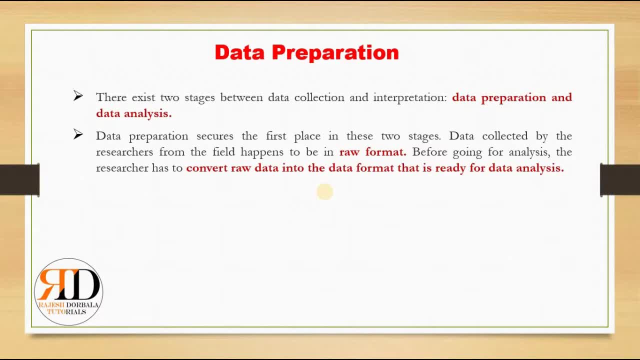 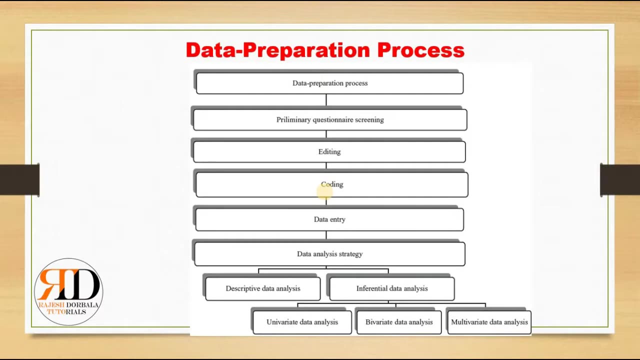 So before going for any analysis and making it friendly for any software, the researcher has to convert raw data into data format that is ready for data analysis. Now data preparation process. So this is an elaborate process. Now data prep. in this one is preliminary questionnaire screening, then editing, coding. 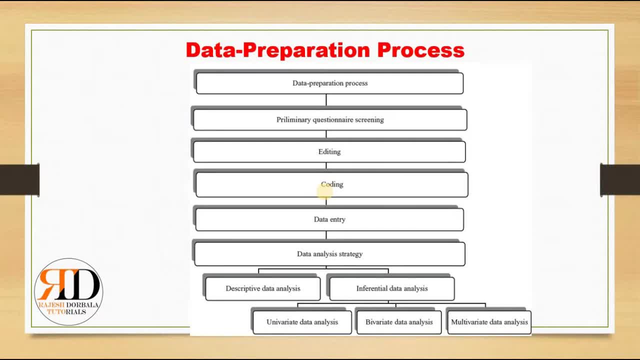 Coding could be like, for instance: if, let us say, I take the gender as male and female, most of the softwares won't recognize male and female. I need to re-code them like, for instance, male could be zero, female could be one or vice versa. 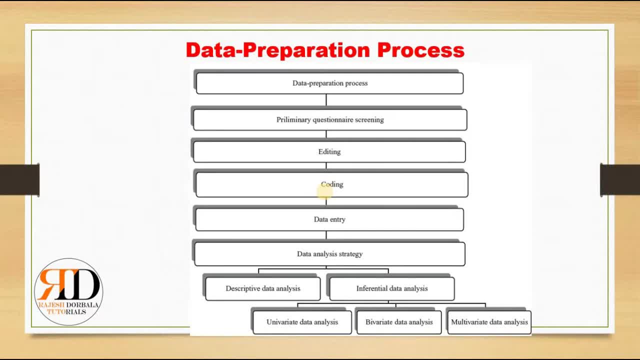 or maybe one or two, anything. So you need to code them. Then data entry. Now this thing: the data collected should be entered into any spreadsheet or any similar thing. Then data analysis strategy. Now I have to develop what kind of analysis strategy should be used. 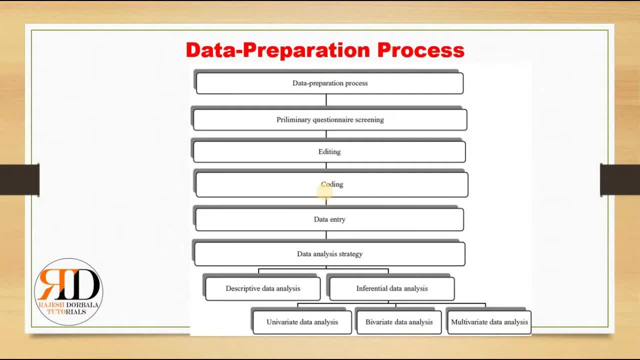 That is, should I use descriptive statistics or descriptive data analysis or inferential data analysis? And if it is descriptive, its things are very simple. But if it is inferential, then again I have to think whether I need to go for univariate or bivariate or multivariate analysis. 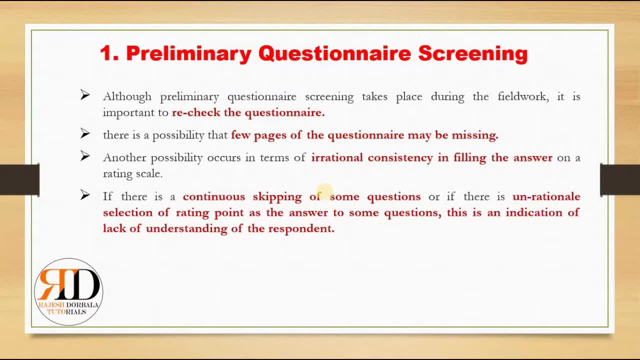 Fine, Now this is the data preparation process. Now, if I explain the step by step that is, first step was preliminary questionnaire screening. That is, I rechecked the questionnaire and there could be possible that few pages of the questionnaire may be missing. 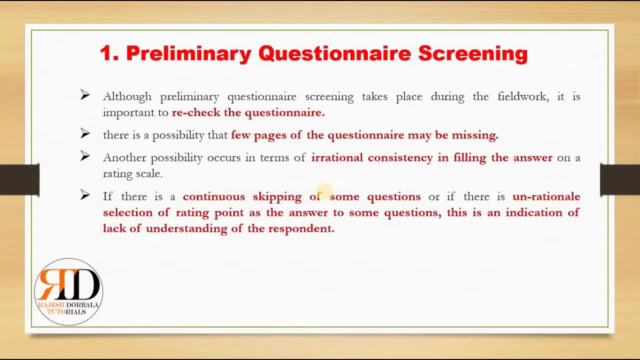 There could be some irrational consistency in filling the answers on rating scale. Maybe some respondents they were not interested in answering and they just kept on rating, you know, 555 or 000 or 333.. So some were either extreme or on the positive side, or extreme on the negative side, or they were neutral. 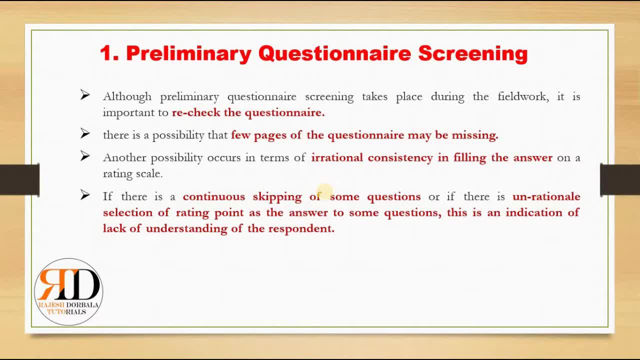 So that is what we mean by there is irrational consistency in filling the answers, And if there is a continuous skipping of some questions, or if there is or there is unrational selection of rating point on answer to some questions, this is an indication of lacking the understanding of the respondent. 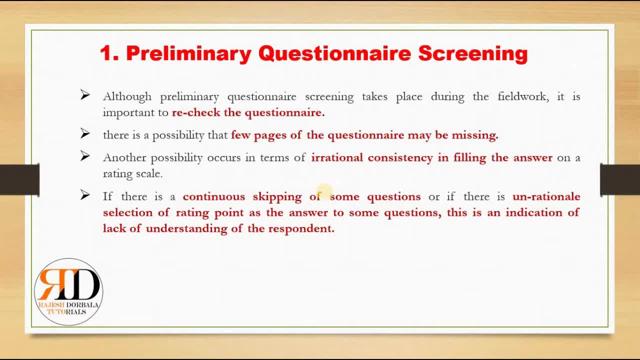 If a respondent. it is quite simple, but let me try to explain or elaborate this Now. it could be possible that a respondent did not respond, Did not understand a question, So the respondent prefers to skip the question. Or there is a possibility that the rating was highly irrelevant. 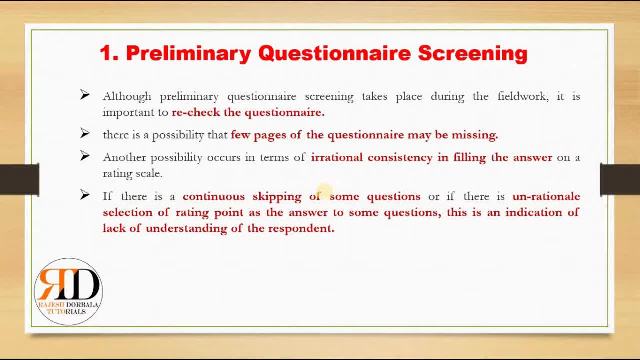 That is to say, the response filled by the respondent is irrelevant or seems irrational, So there is a possibility that the respondent did not understand the question. So this is first: you have to list out, You have to, you know, select all these things where you feel there could be some error in you know. 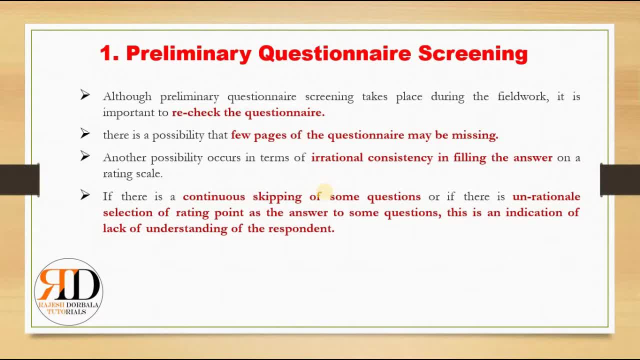 the questionnaire, the design, or maybe there was a printing error, some pages went missing, or maybe the field worker did not administer few pages from the questionnaire, So there could be multiple things. So this is these are the things that are identified during this questionnaire screening. 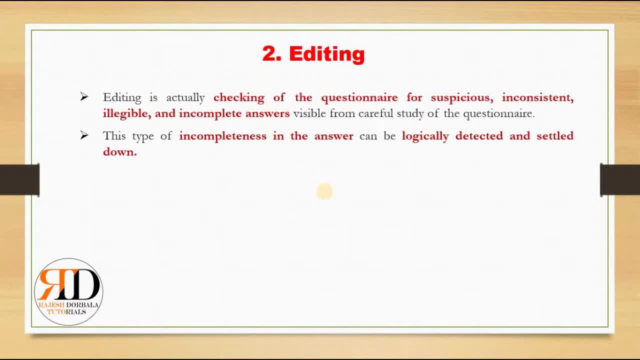 Number 2 is editing. Now editing is actually checking the questionnaire for suspicious, inconsistent, illegible and incomplete answers visible from careful study of the questionnaire. Okay, So again, you check all the, you read all the responses and there could be answers which are illegible. 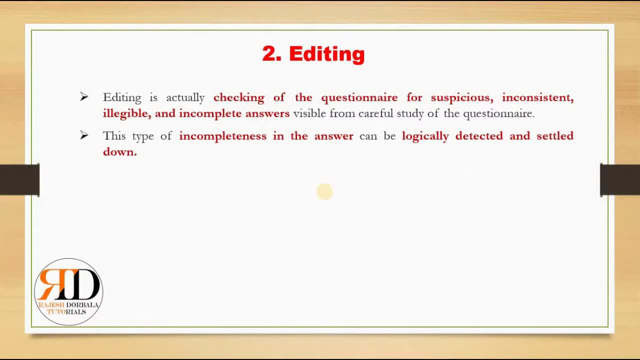 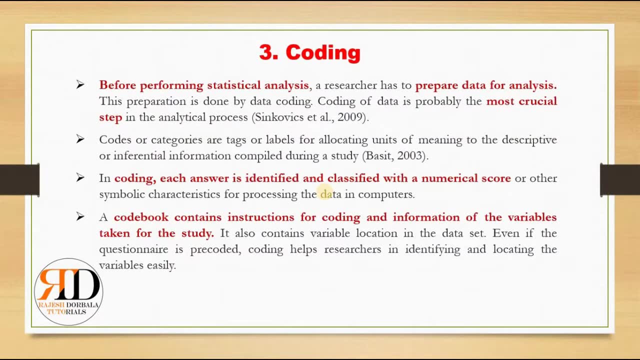 cannot be read or maybe incomplete, Okay, And this type of incompleteness in answers can be logically detected and settled down. Then coding, As I explained, like before performing statistical analysis, a researcher has to prepare data for analysis. This preparation is done by data coding. 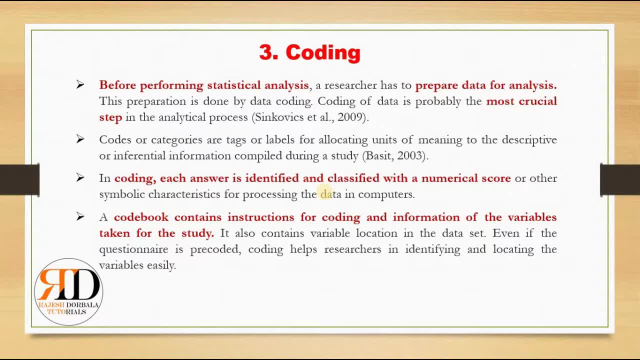 Coding is data. coding of data is probably the most crucial step in analytical process. Now, codes are categories or tags or labels. You know, you convert any kind of categorical variable into factors. Now right, there could be some textual factors which you converted into numeric. 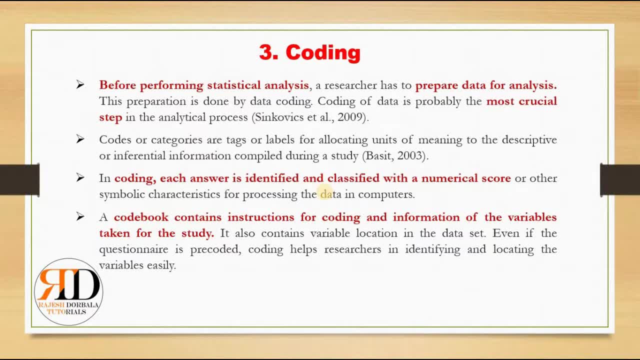 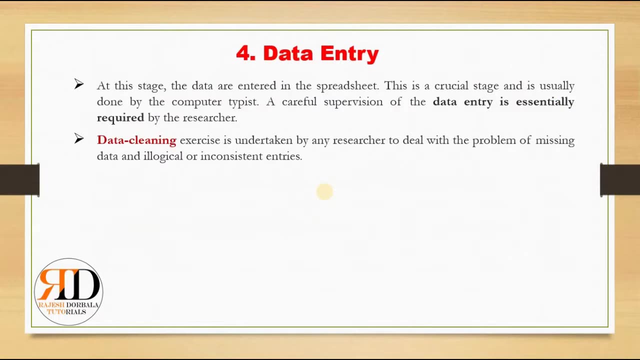 Now a code book contains instructions for coding The information of variables taken for the study. It also contains variable locations in the data set. Even if the questionnaire is pre-coded, coding helps researchers in identifying and locating variables easily. And then comes the task of data entry. 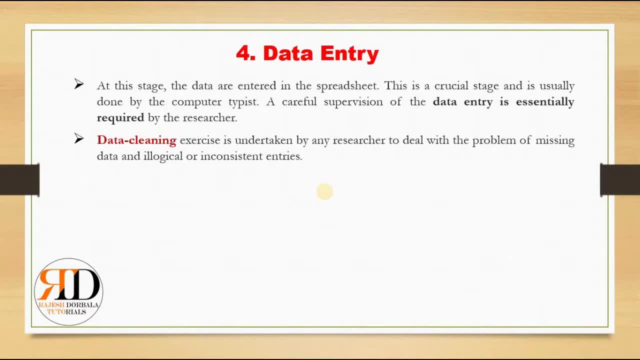 Now, at this stage, the data are entered in a spreadsheet. This is a crucial stage. There shouldn't be any loss in the data or there couldn't be any errors, of omission or confusion. Very careful supervision of data entry is essential, And data cleaning exercise is undertaken by the researcher to deal with the problem of missing data and illogical or inconsistent entries. 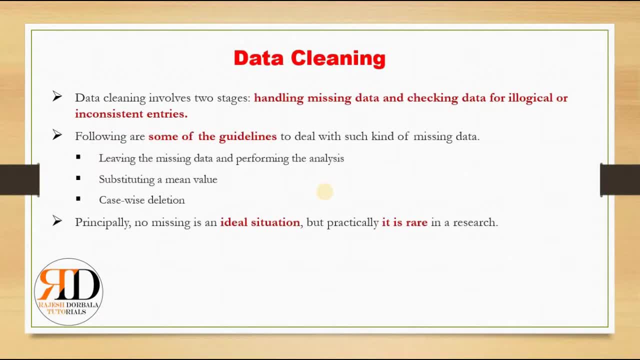 Then, data cleaning, you handle some missing data. There could be some- you know- entries which are out of format. There could be some gibberish entries. So all these things have to be taken care of Now: handling missing data and checking data for illogical or inconsistent entries. 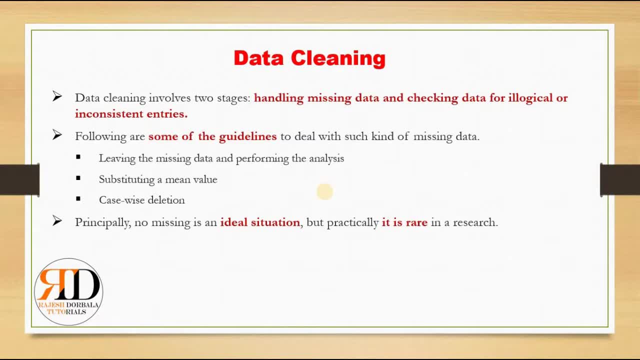 Following are some of the guidelines to deal with missing data: Leaving the missing data and performing the analysis, or substituting a mean value or case-wise deletion. Okay, So, principally, no missing data is an ideal situation, But practically it is rare in research. 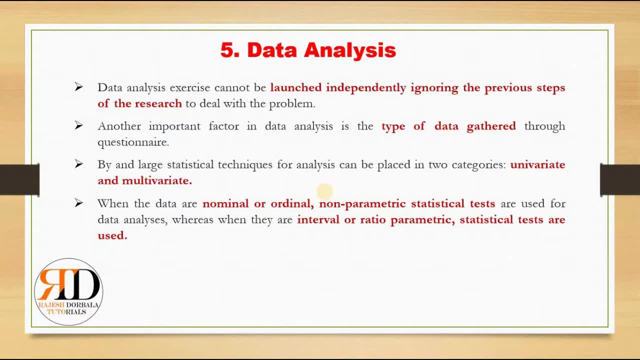 Then you have data analysis. Now, data analysis exercise cannot be launched independently, ignoring the previous steps, So you have to go through all the previous steps in order to reach this stage. Another important factor in data analysis is the type of data gathered through the questionnaire. 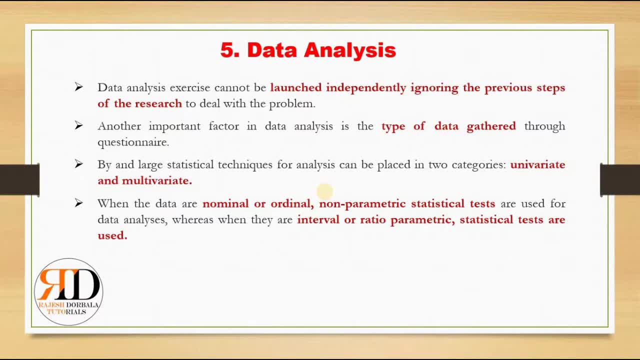 By and large, statistical techniques for analysis can be placed in two categories: univariate and multivariate. Now, when the data are nominal or ordinal, that is, non-parametric statistical tests are used for data analysis, Whereas when they are interval or ratio, statistical tests are used. 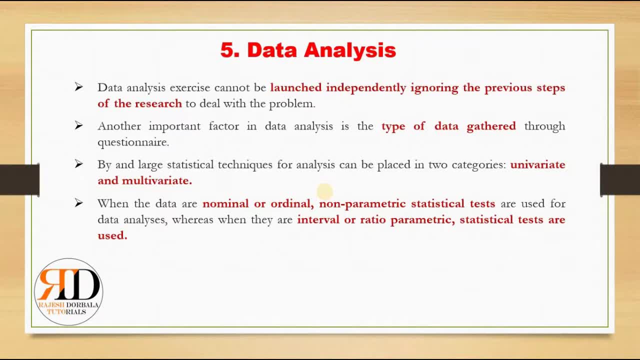 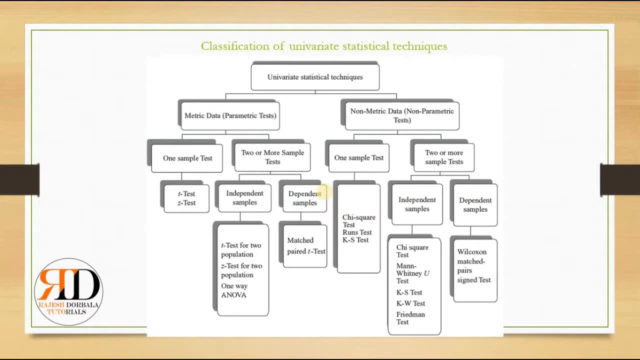 Okay, Statistical or parametric tests are used. Now, these are the classifications of univariate statistical techniques. In univariate, you have metric data. that is parametric or non-parametric. Okay, So if it is metric data, you have parametric tests. 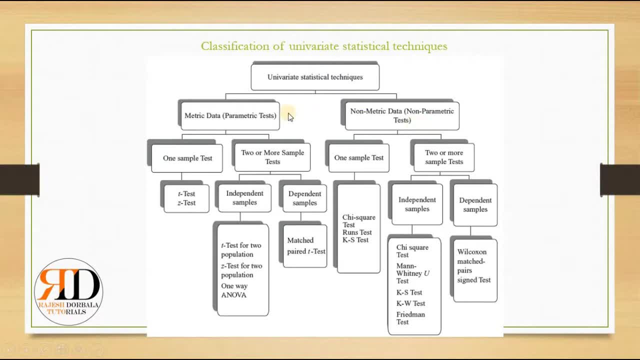 If it is non-metric data, you have non-parametric tests. Metric data is usually in the form of numbers. Non-metric data is usually in the form of characters or string. Now you have to know whether it is a one-sample test or two-sample, two or more-sample test. 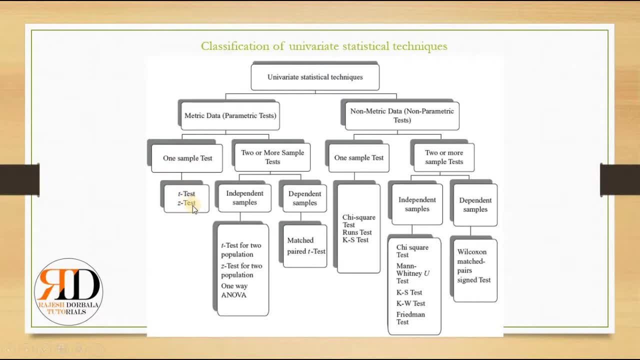 If it is a one-sample test, t-test or z-test is fine. If it is two or more, then if they are independent samples or dependent samples. If they are independent samples, then you can use t-test, That is test for two population. 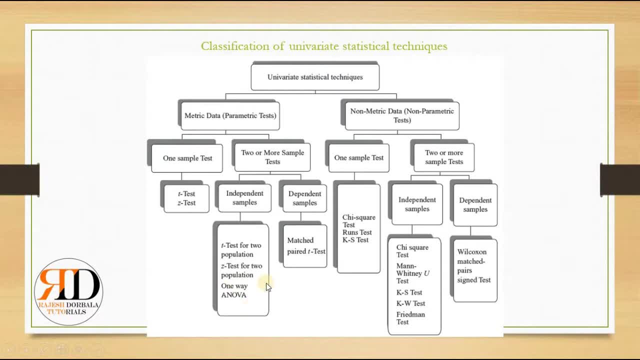 Z-test test for two populations or one-way ANOVA, And if it is a dependent sample, you can use matched paired t-test. And if they are non-parametric tests, then if it is one-sample test or two-sample test. 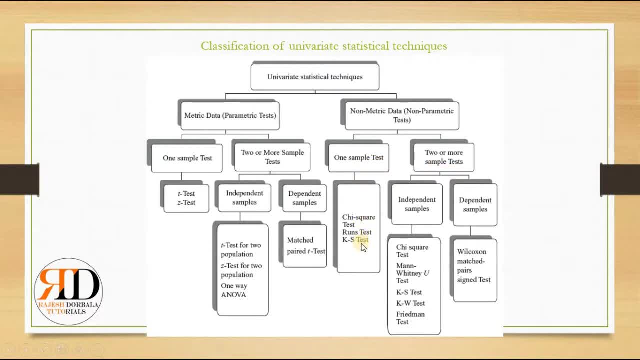 If it is a one-sample test, you can use chi-square test And you can run the KS test, That is Kolmogorov-Smirnov test. Now two or more samples, then independent sample or dependent samples. If they are independent samples, you can use the chi-square test or Mann-Whitney use test or Kolmogorov-Smirnov test. 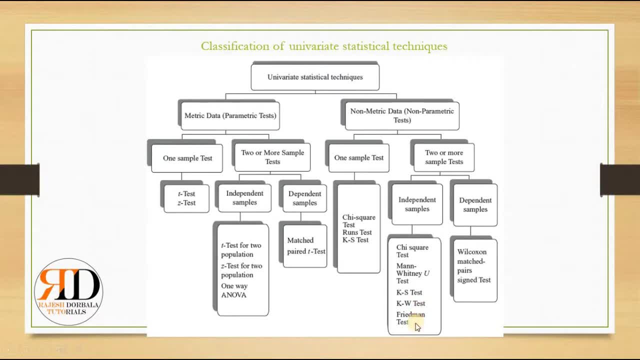 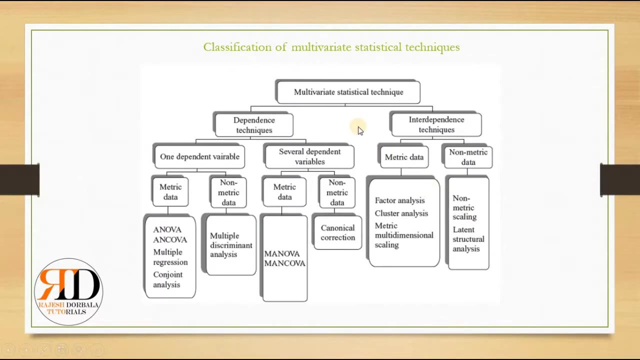 And Kruxow-Wallis test and Friedman test, And if it is dependent samples then you need to have Wilcoxon matched, paired single sign test. Fine, Then classification of multivariate statistical techniques. The multivariate techniques are dependent or independent techniques. 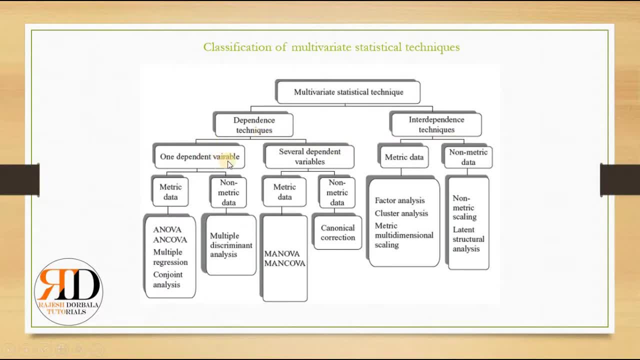 Okay, dependence techniques or independence techniques. One dependent variable, several dependent variables, If it is one dependent. If it is one dependent, you need to figure out whether it is a metric data or non-metric data. Metric data, then you can go for ANOVA, ANCOVA, multiple regression, conjoined analysis. 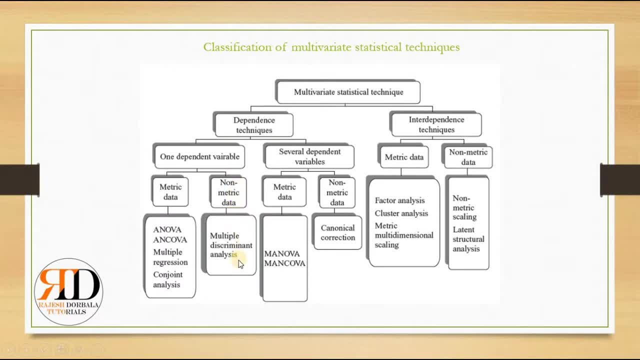 And if it is non-metric data, then you can go for multiple discriminant analysis And then if there are several dependent variables, then metric data, then you can go for MANOVA or ANCOVA Or non-metric tests, then you can go for canonical correction. 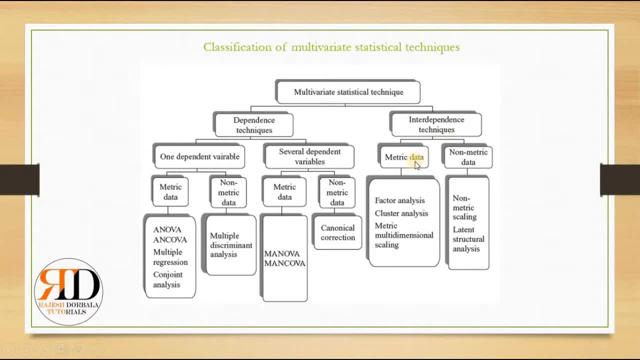 Interdependence techniques, Then you can go for metric data- if it is metric data- or non-metric data. If it is metric data, go for factor analysis, Then cluster analysis, metric multidimensional scaling, that is MMS. And if it is non-metric data, then you can go for non-metric scaling, that is NMS. 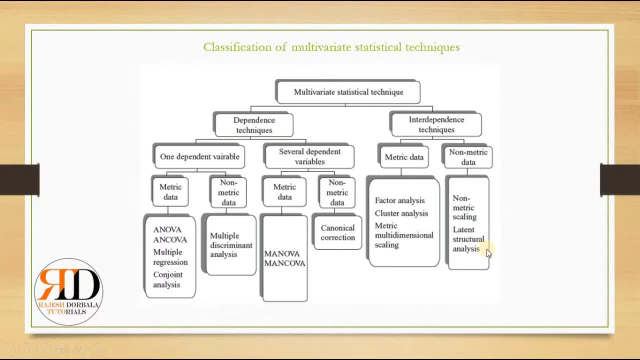 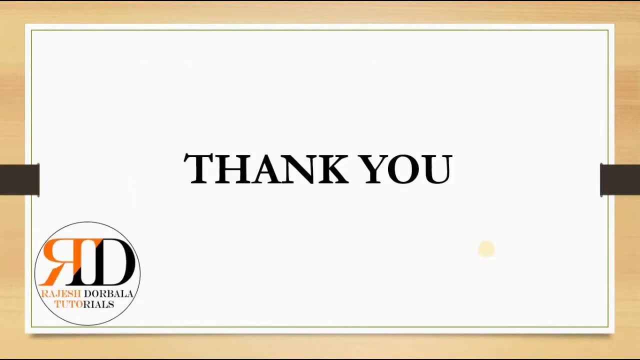 Or latent structural analysis. So these are the classifications of multivariate statistical techniques. Fine, So that was it for today's session. I hope you have a clear understanding of what goes into the fieldwork and how the data is collected, What needs to be taken care of, how you are going to train the staff, that is, the fieldworkers. 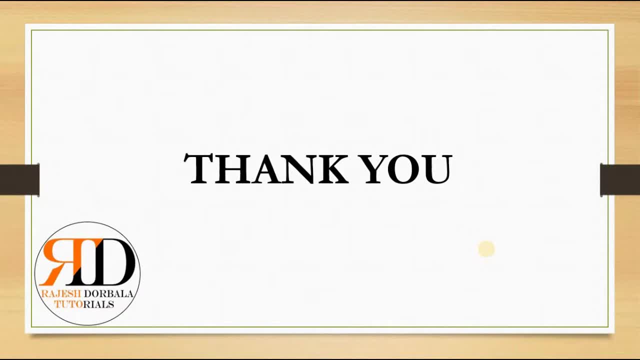 And what you need to do with the data collected. And then what are the various tests that are available and you can apply under various conditions of your data. Fine, See you soon with more detailed lectures on various statistical tests that could be applied on the data that you have collected from your fieldwork. 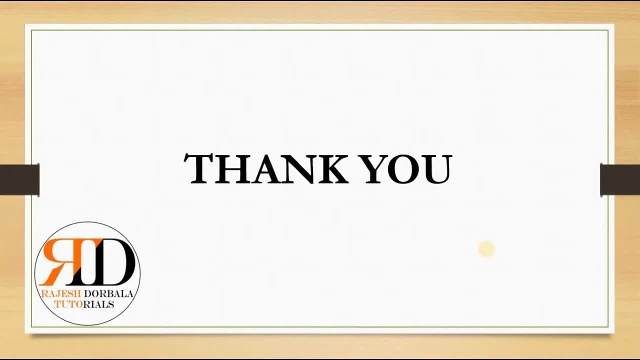 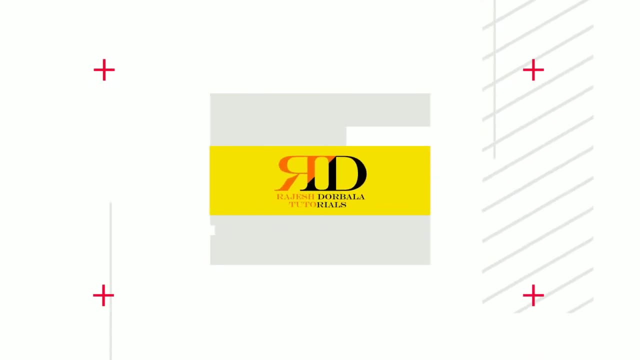 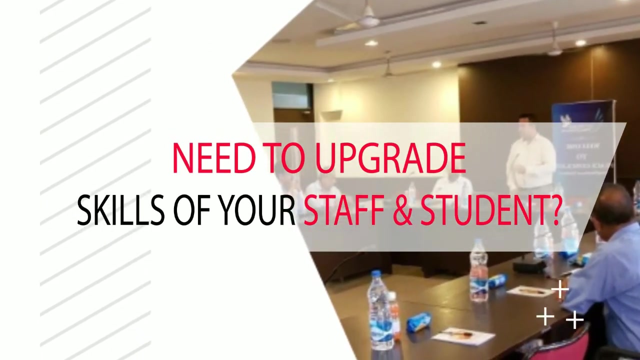 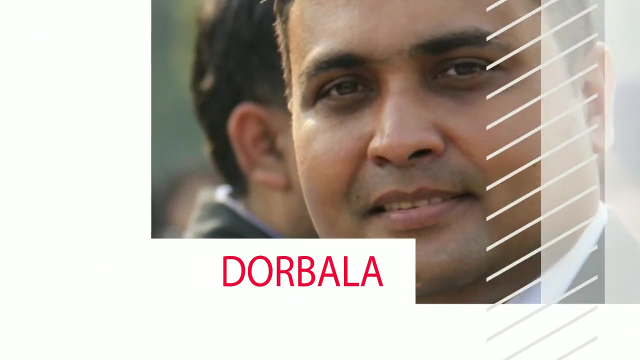 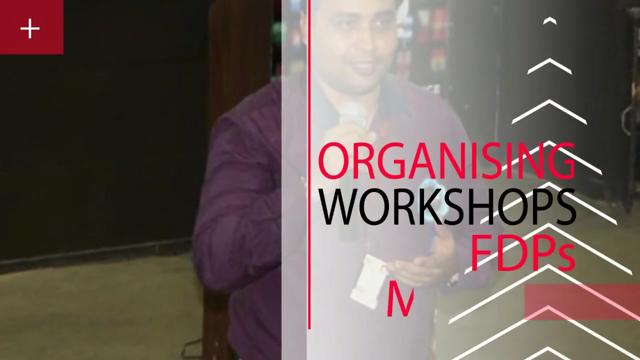 Thank you, See you soon And if you like the videos, please do like it, share it and do subscribe to my channel. Thank you, Thank you, Take care, Bye, Bye, Bye, Bye, Bye, Bye, Bye.